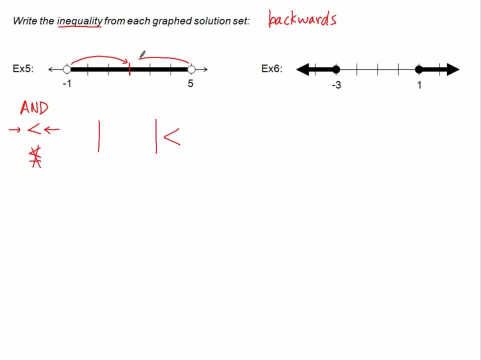 exactly in the middle from one endpoint and the other endpoint. So we could just count out this tick mark. I'm starting here at negative one, so this must be 0 and then 1 and then 2 and then 3 and then 4 and then 5, and that works, If you. 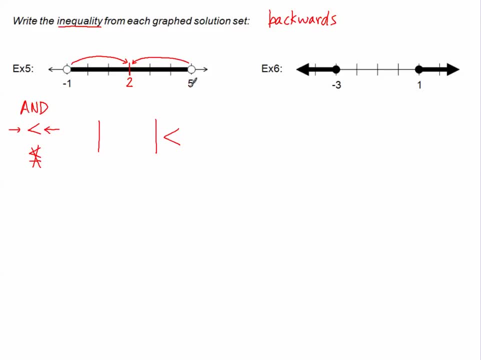 have trouble counting that out. you could take the two endpoints, the negative 1 and the 5, add them together and divide by 2.. That's basically just taking the average of two numbers, which would find the number exactly in the middle. Negative 1 plus 5 is 4.. 4 divided by 2 is 2.. So that's another way to find. 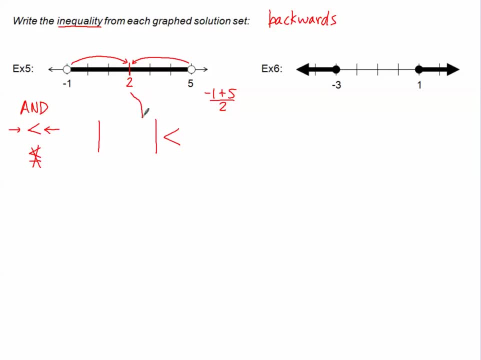 the 2.. Once you know the number that's right in the middle, that's basically like your average, your actual value in the middle. That goes right here. So you're gonna have X minus 2. It's always gonna be X minus that number. that's in. 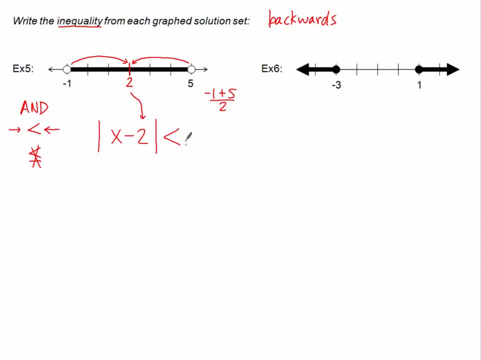 the middle. So great, we have the inside. Now let's figure out what's on the outside. The outside value is always going to be that margin of error, That give or take, Basically the distance from your middle to either one of your endpoints, And clearly you can see that. 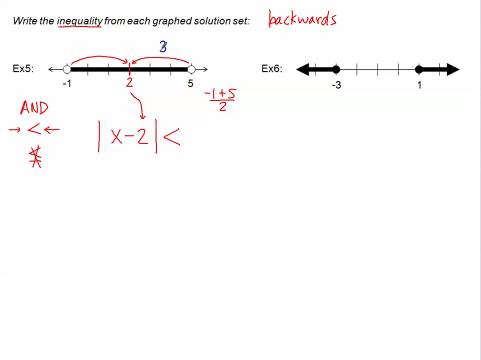 we're counting three tick marks: from 2 to 5 is exactly 3, or from negative 1 to 2 is exactly 3.. It doesn't matter which side we go. There's our margin of error and that number will go right here, And that's it. 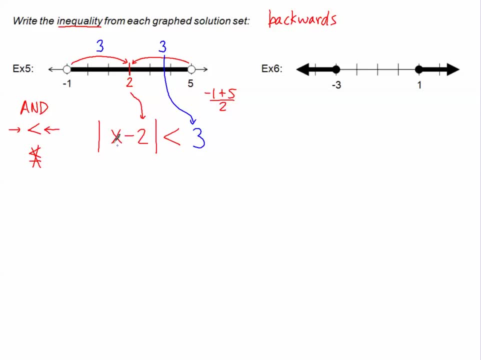 Find the middle number, and it goes in the middle right here. X minus that number. Find the distance between your two points and that number is your margin of error, and it goes out here. Understand how to figure out the symbol and we're finished. We have the absolute value of X minus 2 is less than 3.. Now if for some, 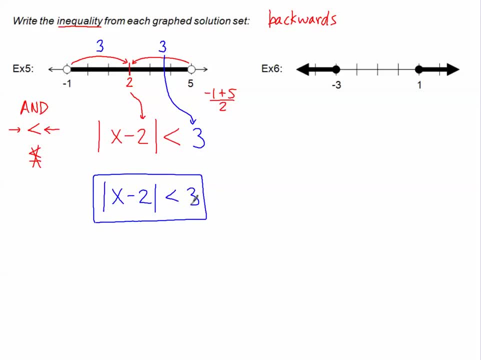 reason you're unsure if you are correct or not. Some people tend to mix up the two numbers. You can always solve what you think. your answer is: Solve it And see if your graph solution set is exactly this. On our state test, when 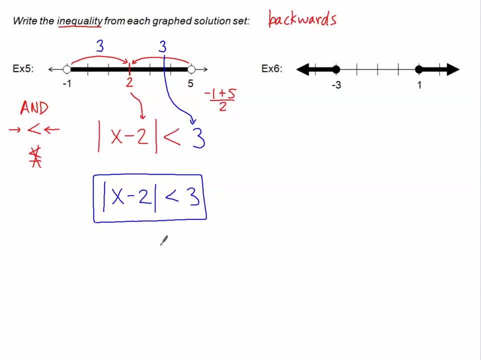 they're asking you to do these backwards problems. they're going to give you four answer choices. You could solve each one of the answer choices and see which one is the graph And you could sort of go forwards on their backwards problem. Let's see if you understood all that and try it with the second example. So this 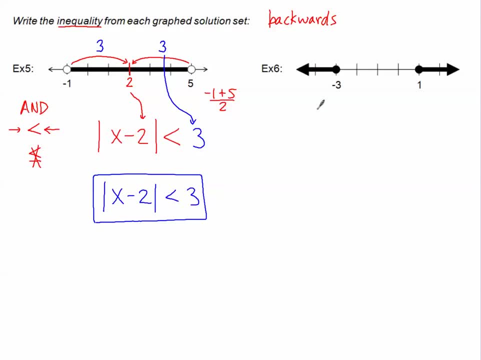 is our OR statement. I know that this is OR. I sort of think of you, not to draw this- but if you think of your like in a boat, like in a rowboat, and you're rowing across the lake, The ors are on the outside. 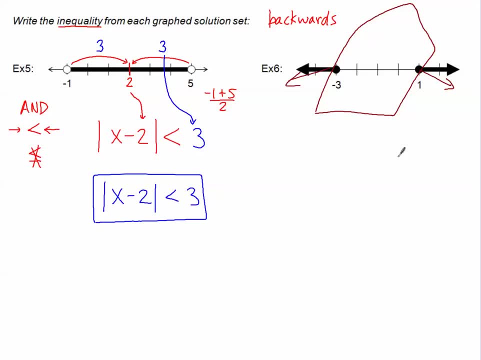 of your boat, and that's how I like to think of the or statement. I'm going to undo all that, but that was a fun visual, if you like, that Sort of a play on words, of the word or that we use in a rowboat. This is an or statement, and if it's an or, we're using greater than or greater than. 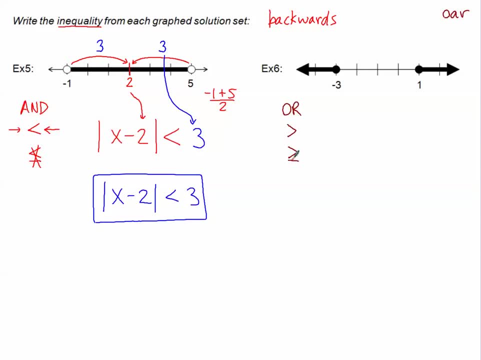 or equal to. So I know it's got to be one of these two. Now, since I see these closed circles, I must be including the values, so I'm not using that one. This must be the symbol that I'm using. The absolute value of something is going to be greater than or equal to, something else. 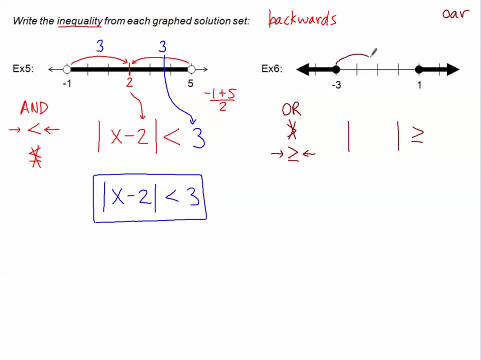 Now let's go see if we can find those somethings. I guess We're going to find the number that's right in the middle, That tick mark right there: Negative, three negative, two negative 15.. 1 0, 1. yep, it works. or you could take that negative 3 and the 1, add them together and divide by 2. 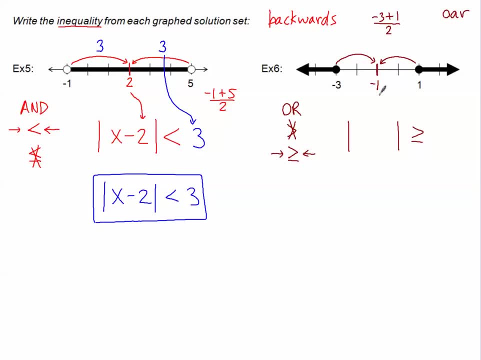 that's another way to figure out that. you've got negative 1 right in the middle. that's going to go right here: x minus negative 1. now, obviously we're not going to leave it like this. i'll clean this up in my next step. but it's always x minus whatever this number is, if it happens to be negative, we'll. 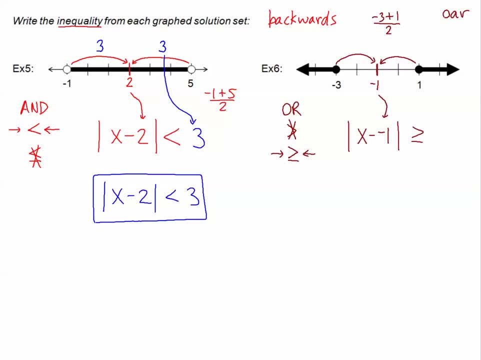 deal with that, and then the other part of this. i have to find how much distance there is between the middle and the end point, and you can clearly see that there are two tick marks. so it must be the value of 2 and that goes right here. that's your, your give or take, your margin of error. so